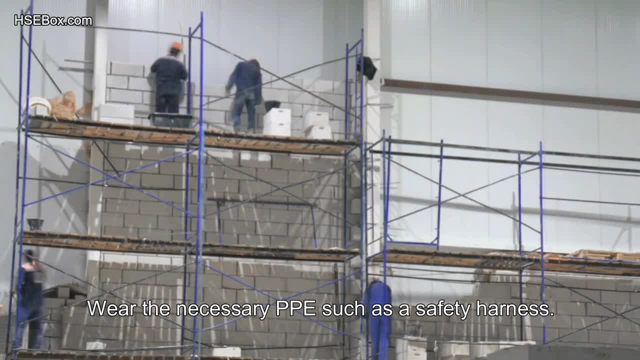 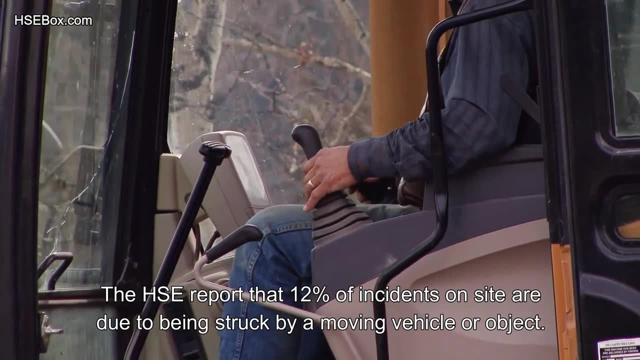 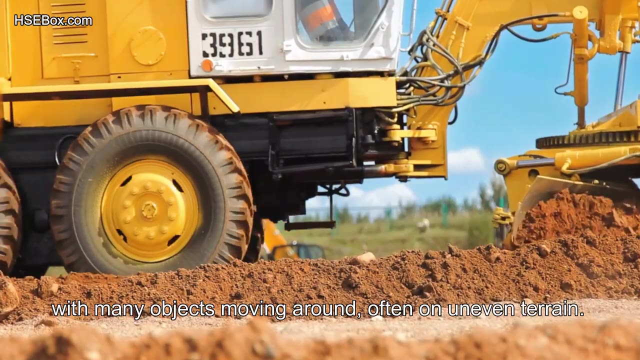 Wear the necessary PPE, such as a safety harness Number 2.. Moving Objects: The HSE report that 12% of incidents on site are due to being struck by a moving object. A construction site is an ever-changing environment With many objects moving around, often on uneven terrain. 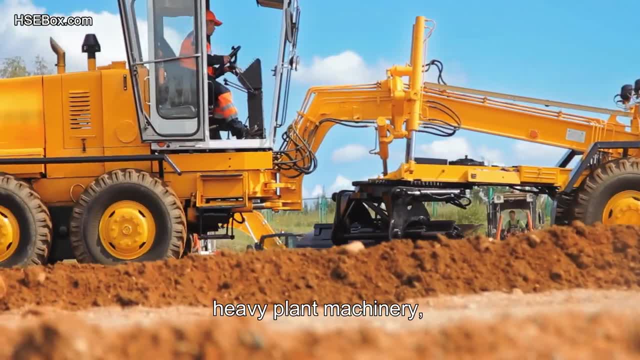 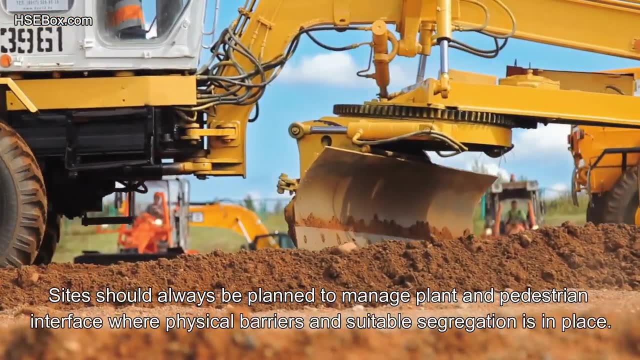 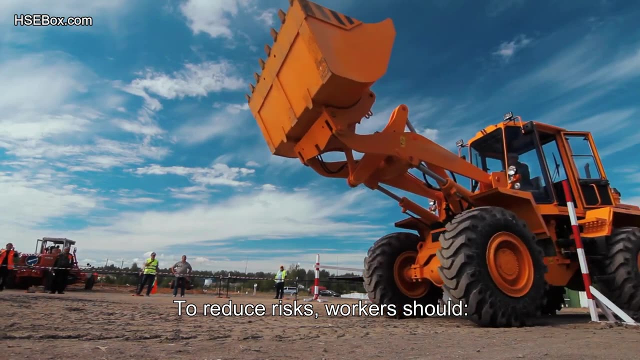 Delivery vehicles, heavy plant machinery and overhead lifting equipment pose a hazard to site workers and operators. Sites should always be planned to manage plant and pedestrian interface, where physical barriers and suitable segregation is in place To reduce risks. workers should Never stand in line. 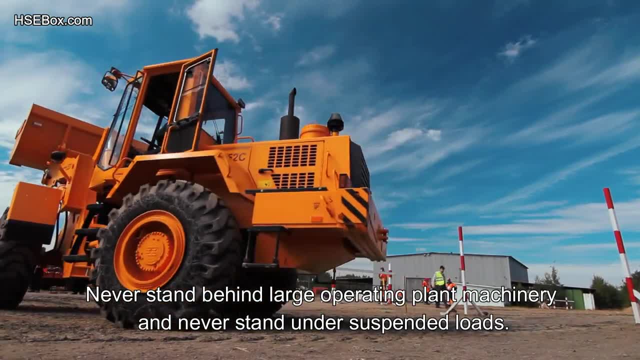 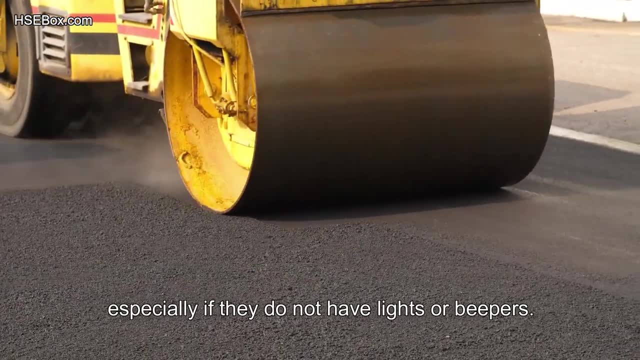 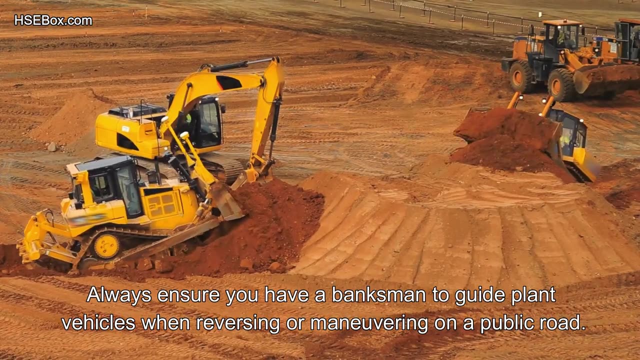 Never stand behind large operating plant machinery and never stand under suspended loads. Avoid working close to moving objects and be careful of their surroundings, Especially if they do not have lights or beepers. Always ensure you have a banksman to guide plant vehicles when reversing or maneuvering on a public road. 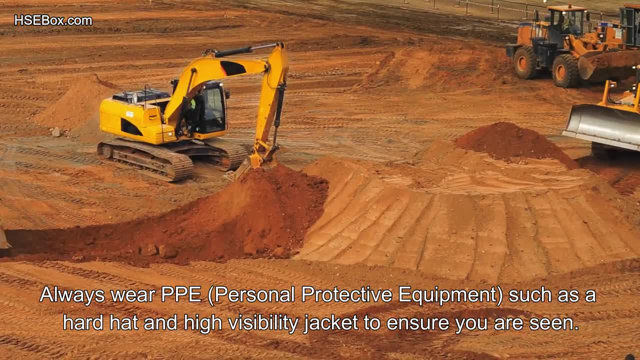 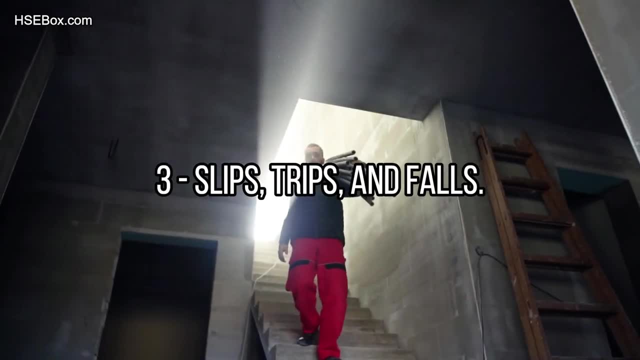 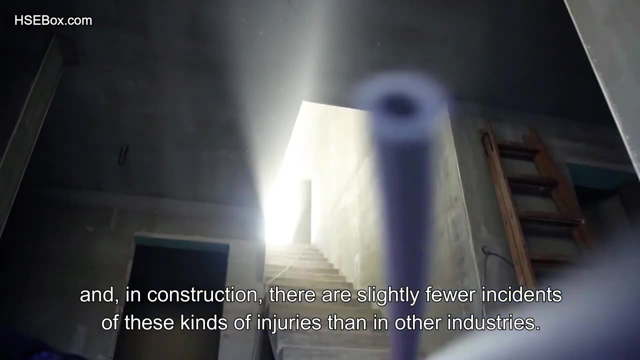 Always wear PPE personal protective equipment such as a hard hat and high visibility jacket to ensure you are seen. Number 3. Slips, Trips and Falls. Slips, trips and falls can happen in almost any environment, And in construction there are slightly fewer incidents of these kinds of injuries than in other industries. 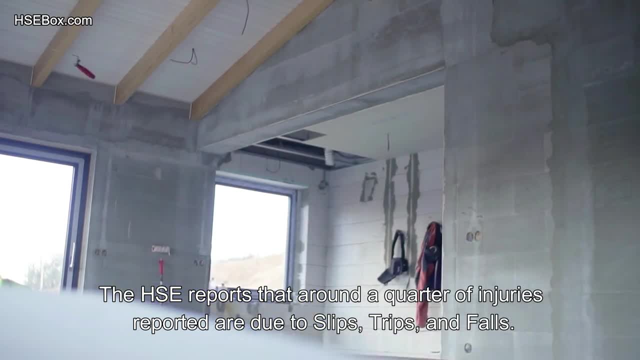 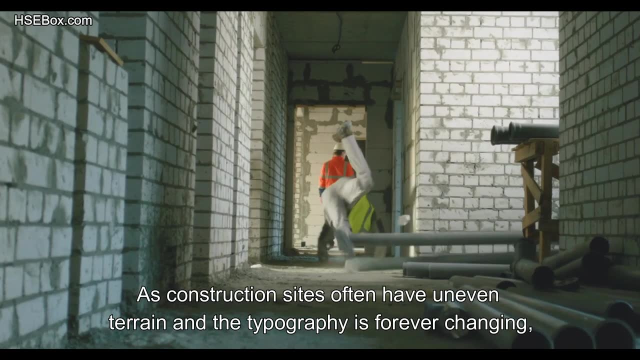 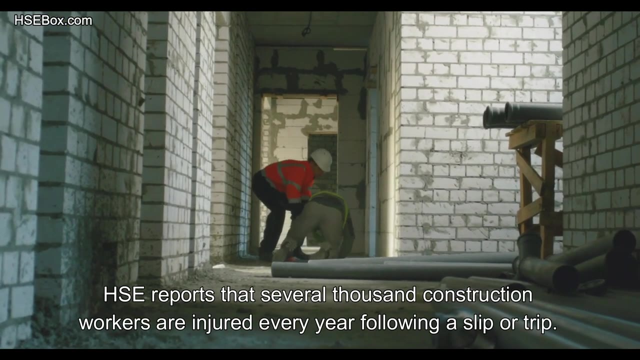 The HSE reports that around a quarter of injuries reported are due to slips, trips and falls. As construction sites often have uneven terrain and the typography is forever changing, it is unsurprising that slips, trips and falls are common hazards. HSE reports that several thousand construction workers are injured every year following a slip. 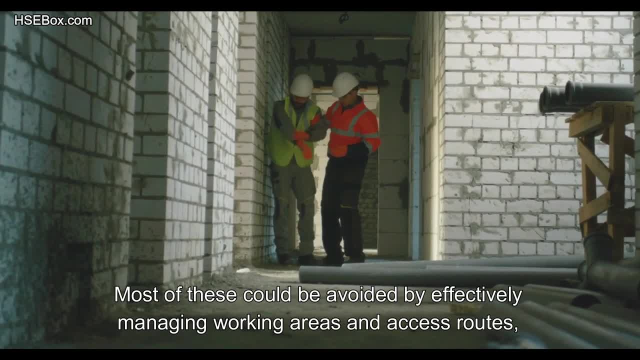 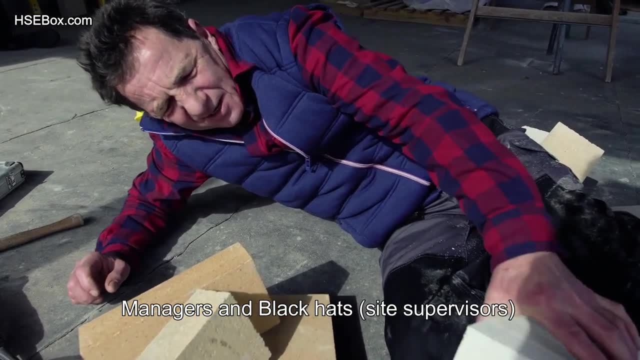 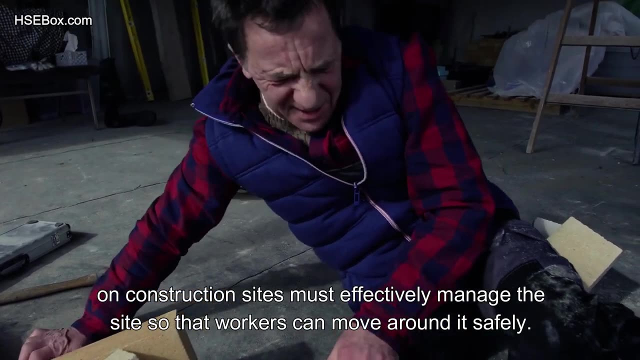 or trip. Most of these could be avoided by effectively managing working areas and access routes such as excavations and footpaths. Managers and black hats- site supervisors on construction sites must effectively manage the site so that workers can move around it safely. 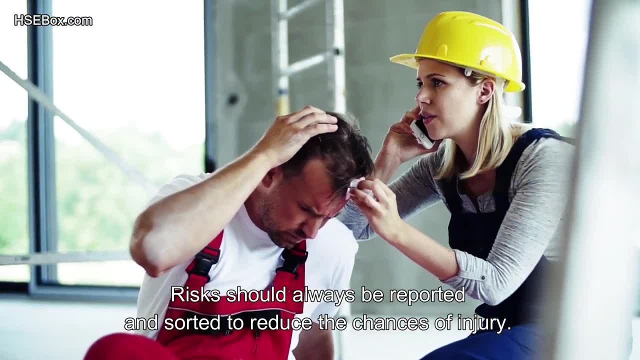 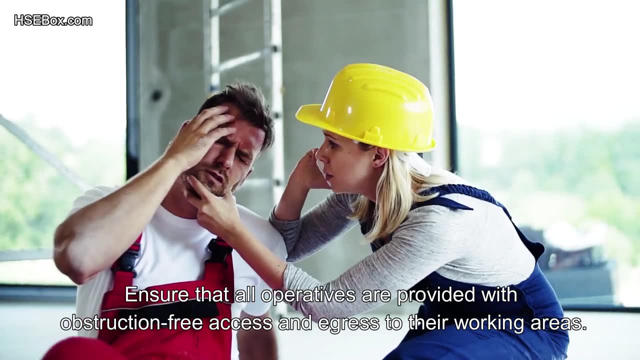 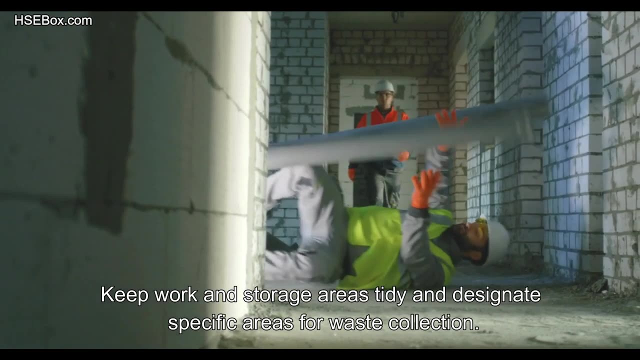 Risks should always be reported and sorted to reduce the chances of injury. To reduce harm due to slips, trips and falls, you should ensure that all operatives are provided with obstruction-free access and egress to their working areas, Keep work and storage areas tidy and designate specific areas for waste collection. 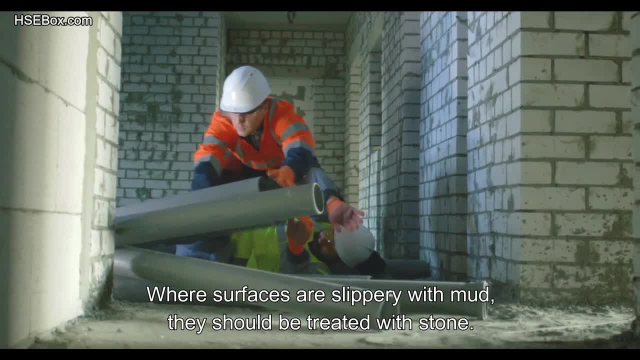 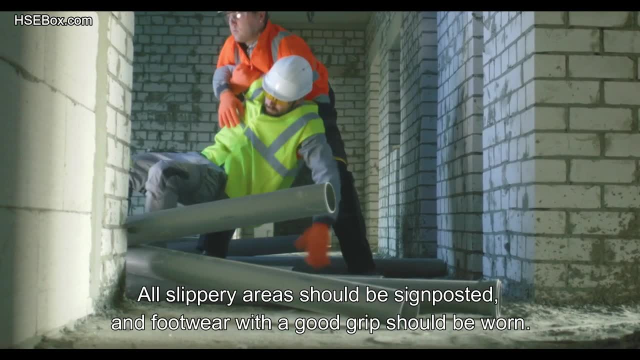 Where surfaces are slippery with mud, they should be treated with stone. Where surfaces are slippery with ice, they should be treated with grit. All slippery areas should be signposted and footwear with a good grip should be worn. Number 4. Noise. 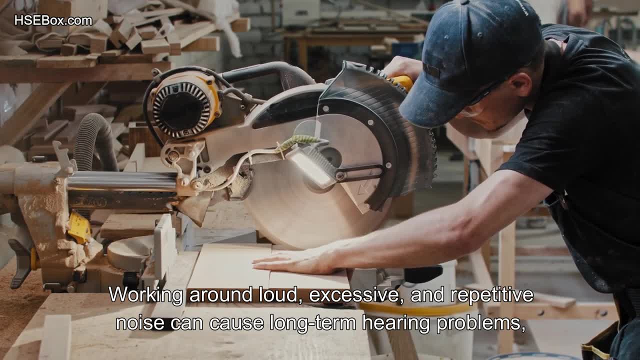 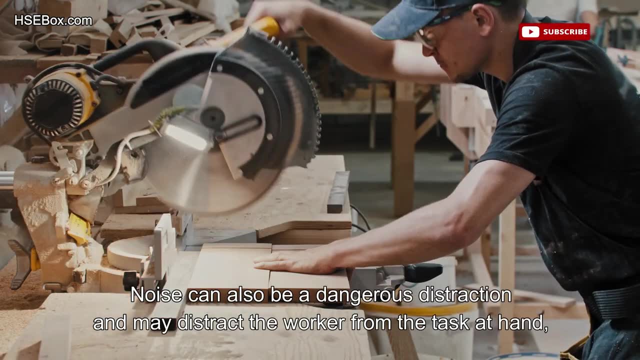 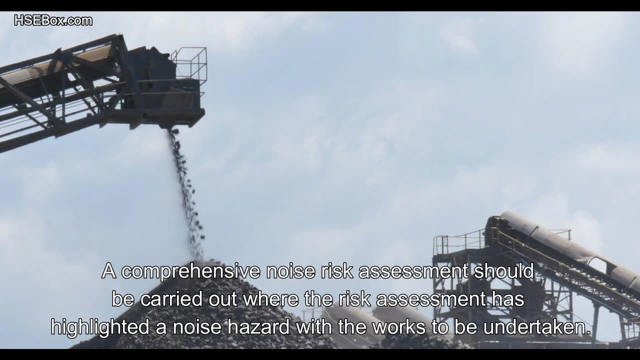 Working around. loud, excessive and repetitive noise can cause long-term hearing problems such as deafness. Noise can also be a dangerous distraction and may distract the worker from the task at hand, which can cause accidents. A comprehensive noise risk assessment should be carried out. where the risk assessment has highlighted a noise hazard, with the works to. 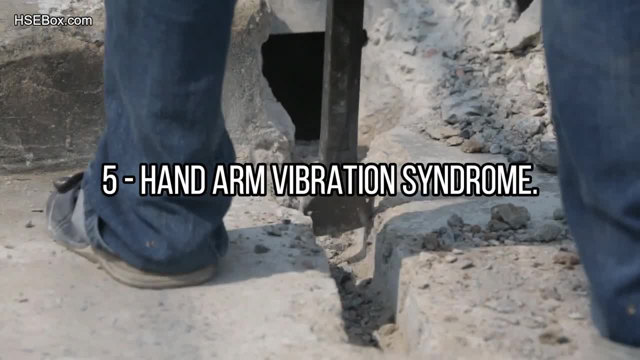 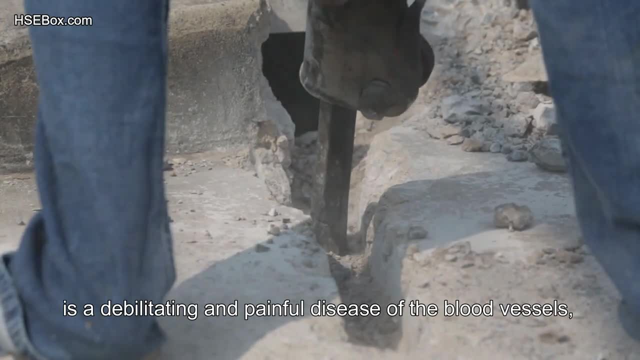 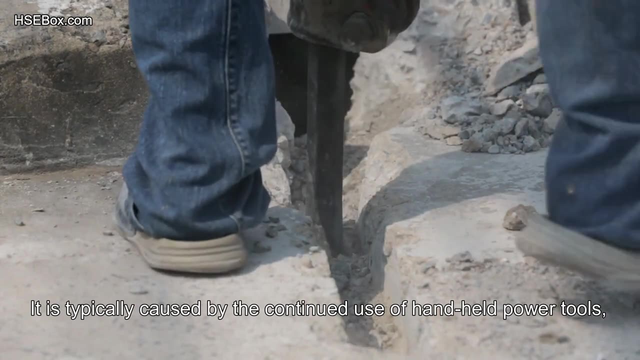 be undertaken. Number 5. Hand-arm vibrations Syndrome- Halves. Hand-arm vibration syndrome is a debilitating and painful disease of the blood vessels, nerves and joints. It is typically caused by the continued use of handheld power tools, including vibratory power tools and ground working equipment. 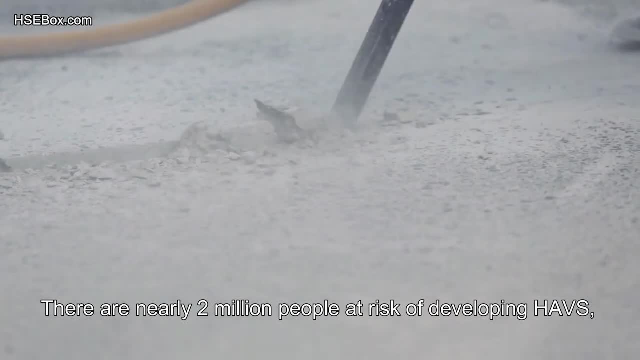 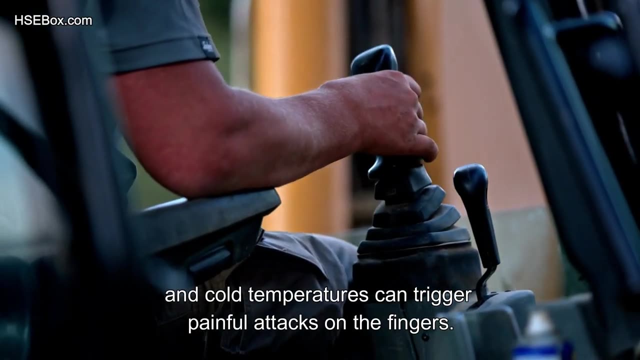 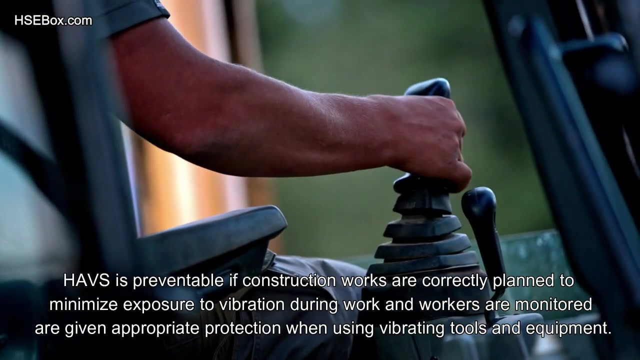 There are nearly 2 million people at risk of developing halves, resulting in the inability to do fine work, and cold temperatures can trigger painful attacks on the fingers. Once the damage is done, it is permanent. Halves is preventable if construction works are correctly planned to minimize exposure to. 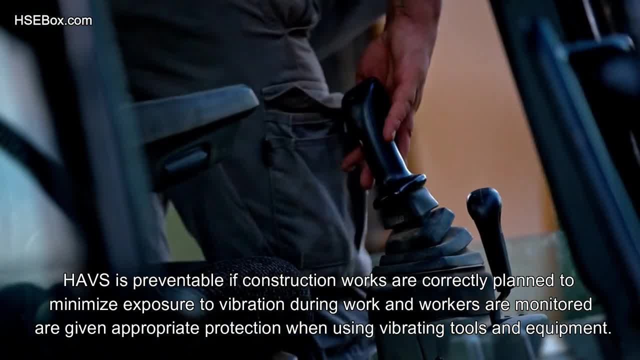 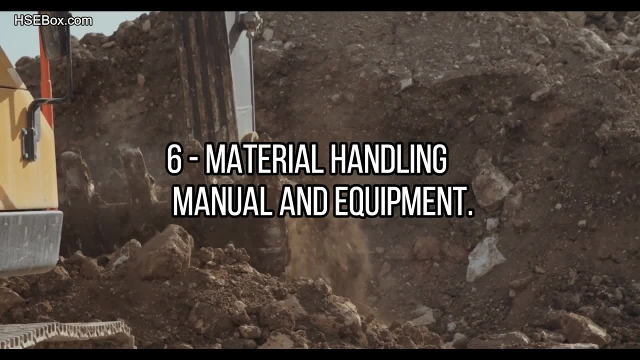 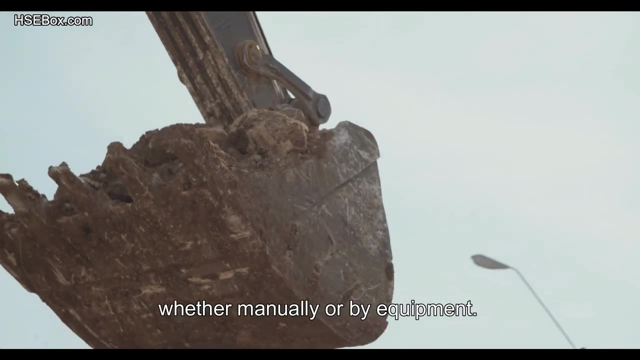 vibration during work and workers are monitored, are given appropriate protection when using vibrating tools and equipment. Number 6. Material handling, manual and equipment. Materials and equipment are constantly being lifted and moved around construction sites, whether manually or by equipment. Either way handling carries a degree of risk. 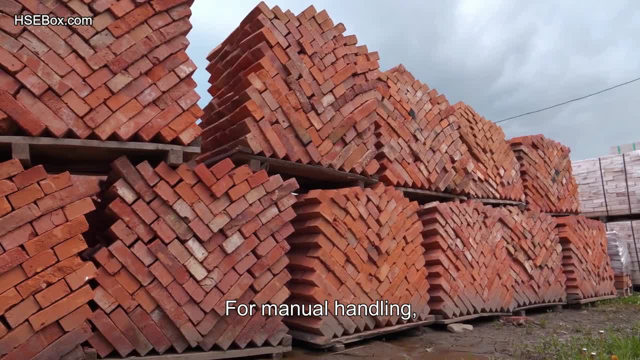 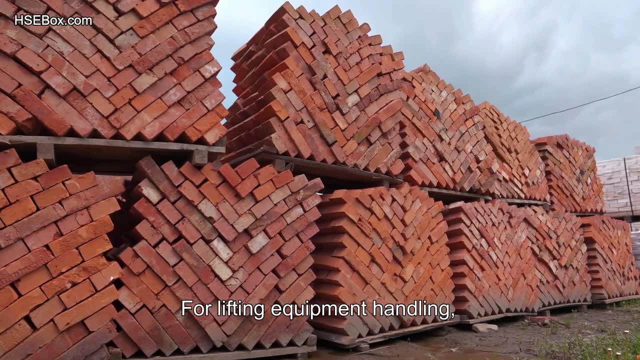 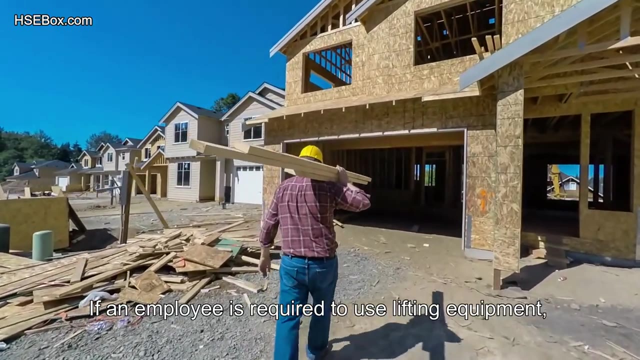 For manual handling, training must be provided to ensure employees can lift and carry materials safely. For lifting equipment handling, there are lots of risks, especially when operating lifting equipment on uneven ground. If an employee is required to use lifting equipment, they must be trained to. 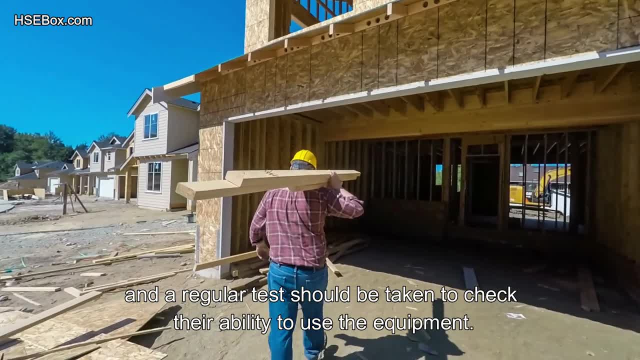 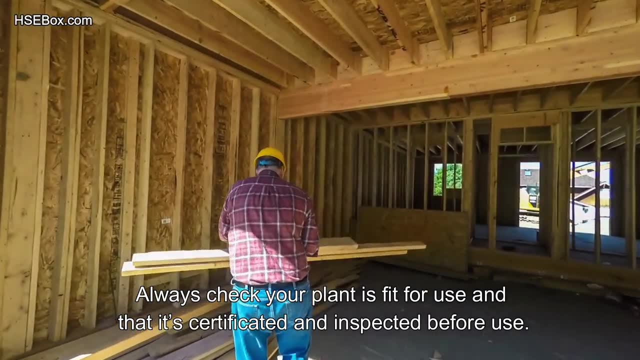 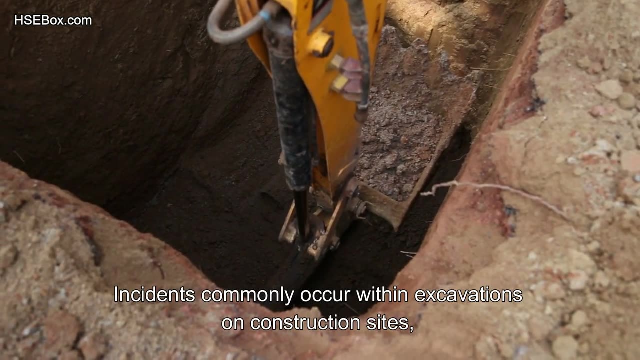 operate the equipment safely and a regular test should be taken to check their ability to use the equipment. Always check your plant is fit for use and the equipment is safe to use. Number 7. Excavations. Incidents commonly occur within excavations on construction sites. 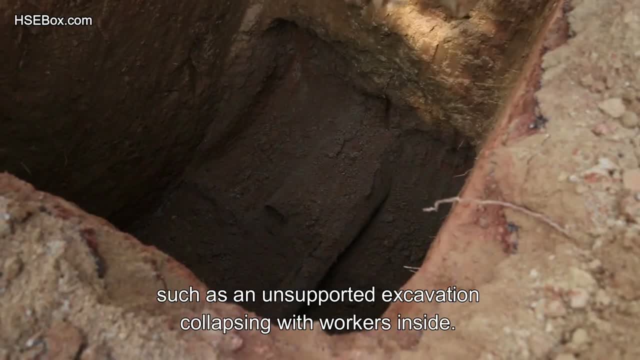 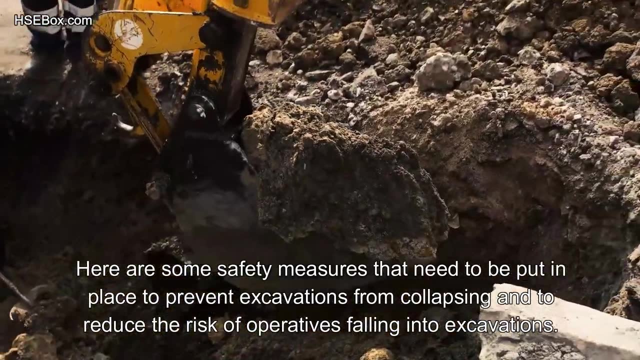 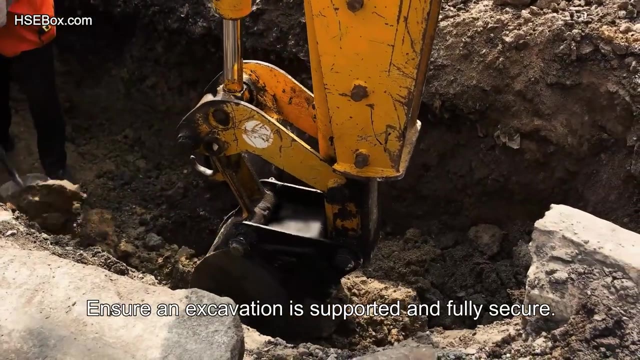 such as an unsupported excavation collapsing with workers inside. Here are some safety measures that need to be put in place to prevent excavations from collapsing and to reduce the risk of operatives falling into excavations. Never work in an unsupported excavation. Ensure an excavation is supported and inspected before use. 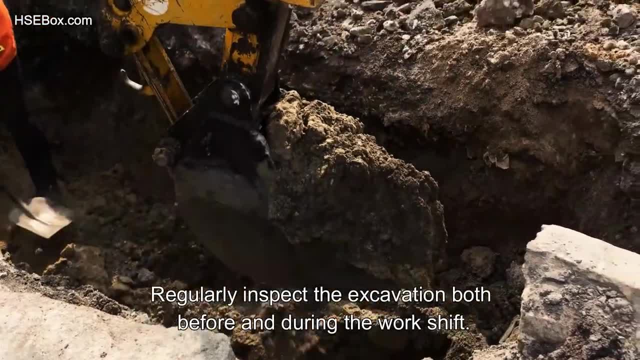 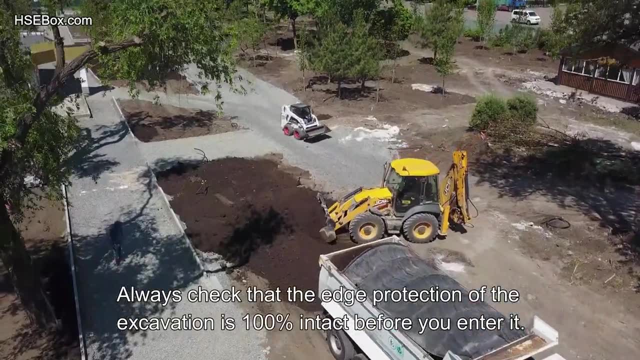 Ensure an excavation is supported and inspected before use. Ensure an excavation is supported and fully secure. Regularly inspect the excavation both before and during the work shift. Always check that the edge protection of the excavation is 100% intact before you enter it. 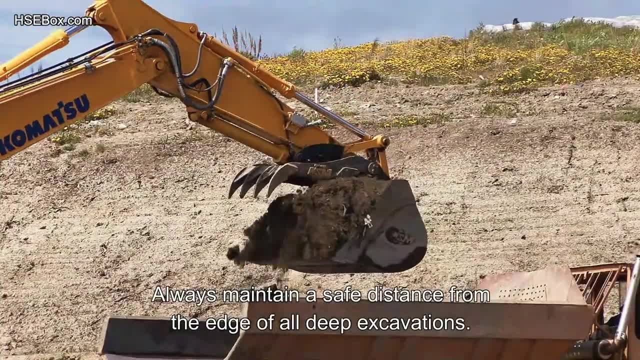 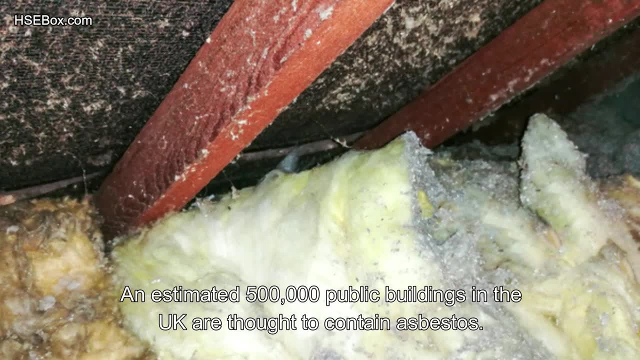 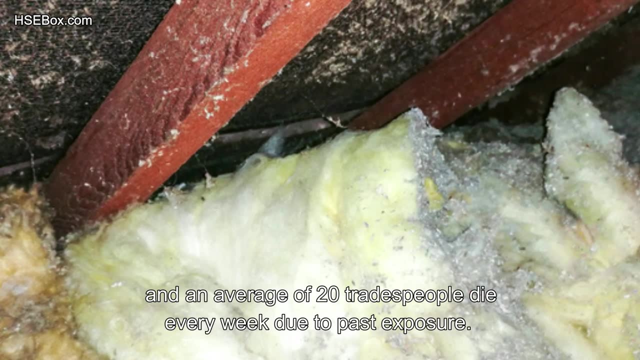 Always maintain a safe distance from the edge of all deep excavations. Number 8. Asbestos. An estimated 500,000 public buildings in the UK are thought to contain asbestos. Asbestos kills around 5,000 workers per year and an average of 20 tradespeople die every week due to past exposure. 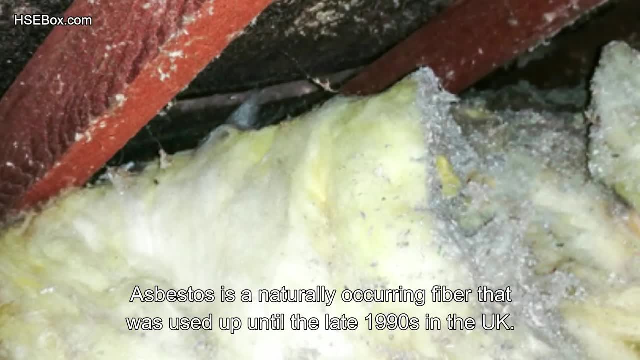 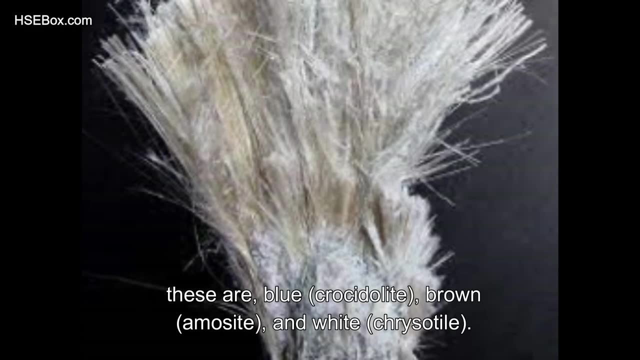 Asbestos is a naturally occurring fibre that was used up until the late 1990s in the UK. There are three types of asbestos fibres commonly used in the UK. These are blue crossitalite, brown amazate and white chrysotile. 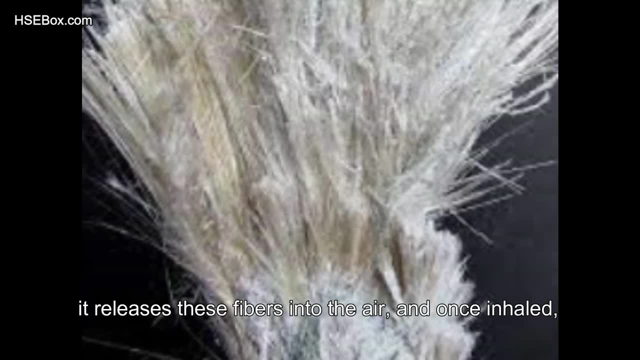 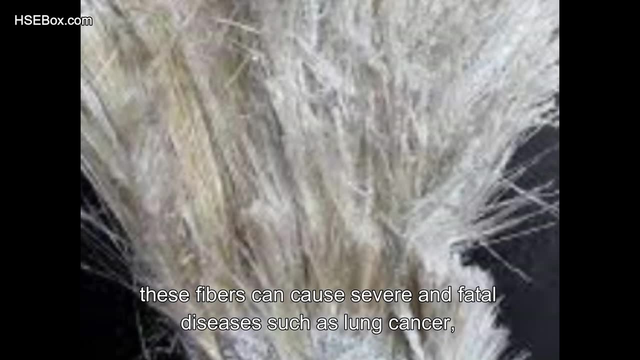 When asbestos is damaged, it release these fibres into the air and, once inhaled, these fibres can cause severe and fatal diseases, such as lung cancer, asbestosis and pleural thickening. Workers on construction sites must be trained to understand what to do. 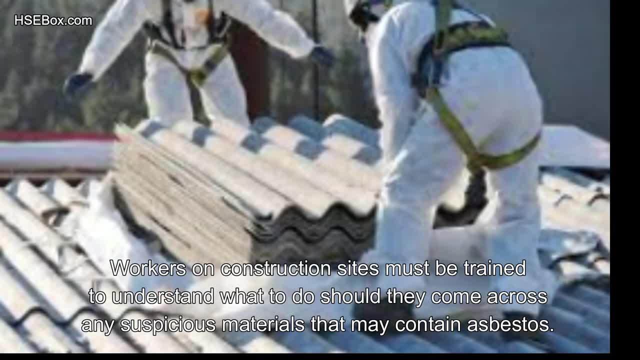 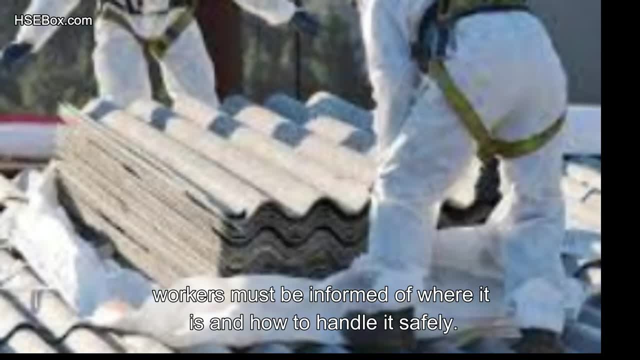 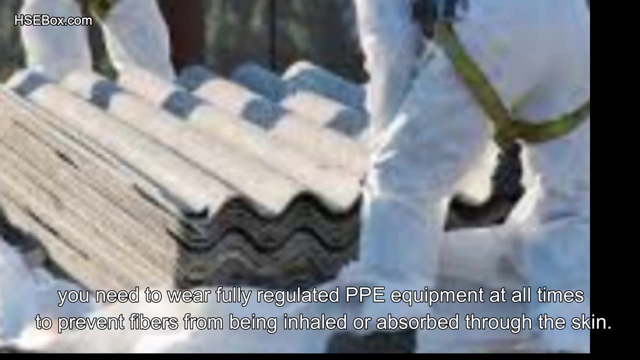 should they come across any suspicious materials that may contain asbestos. If there is asbestos on the construction site, workers must be informed of where it is and how to handle it safely. When handling asbestos, you need to wear fully regulated PPE equipment at all times to prevent fibres from being inhaled. 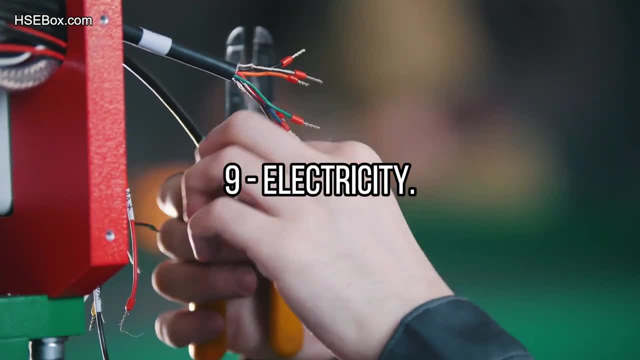 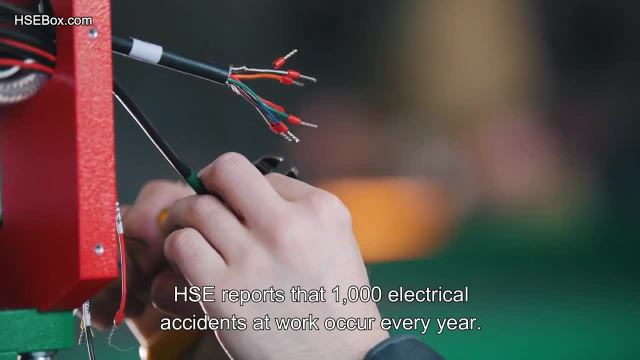 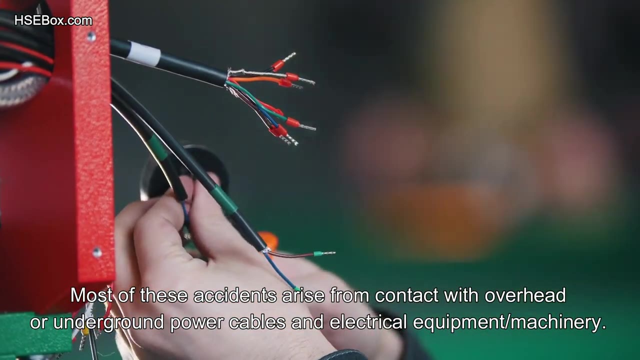 or absorbed through the skin. HSE reports that 1,000 electrical accidents at work occur every year. Most of these accidents arise from contact with overhead or underground power cables and electrical equipment-slash-machinery. In civil engineering, strikes against services are common. 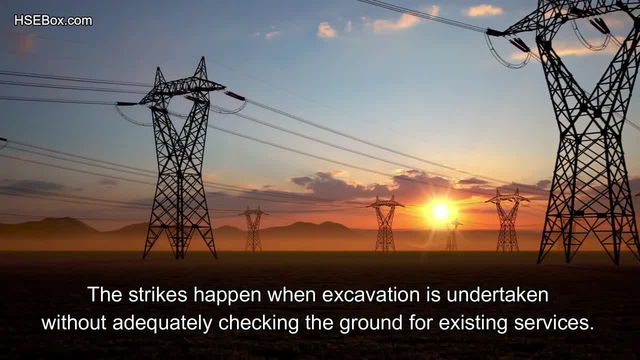 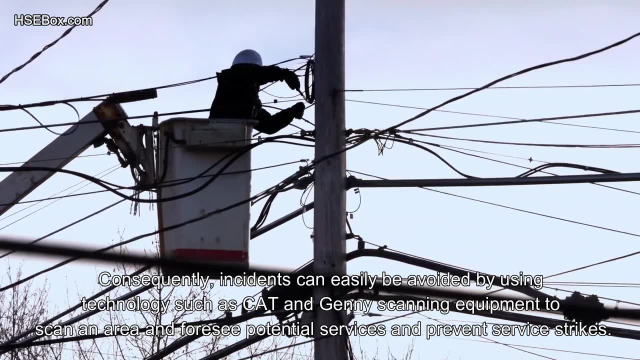 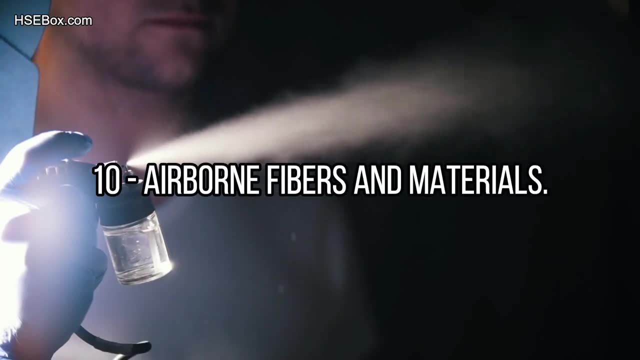 The strikes happen when excavation is undertaken without adequately checking the ground for existing services. Consequently, incidents can easily be avoided by using technology such as CAT and GENI scanning equipment to scan an area and foresee potential services and prevent service strikes. Number 10, Airborne Fibres and Materials.